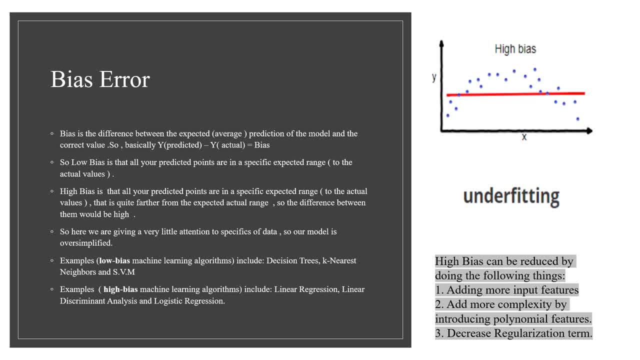 so, um, here we are actually giving very less attention to the specifics of the data, so our model is oversimplified. as you can see in the in the graph here, our model is just a simple line that's spanning over this data points, while it should not be like this. it's very simplified model. 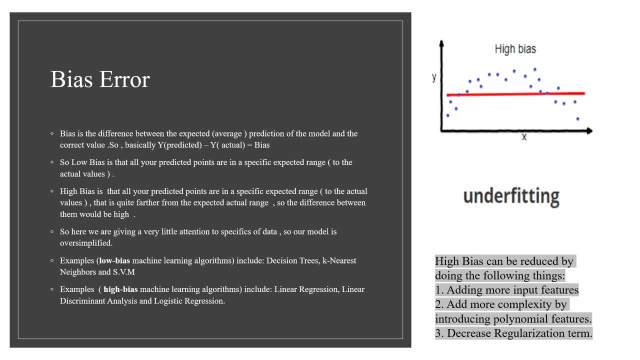 so that's what the one of the thing that's says that you know this. your model has got high bias and the examples would be: uh- low bias, machine learning algorithm state, which include uh decision trees k near knn and svm. those are the examples with uh. 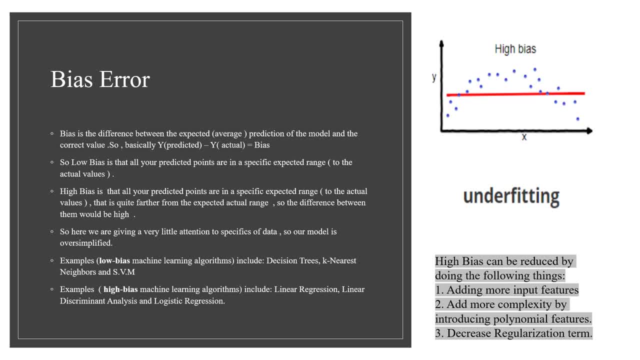 low bias and um and that algorithms which are high bias. they include, uh, linear regression, linear discriminant analysis and logistic regression. okay, which is this thing is also called as underfitting. you know you are oversimplifying your algorithm there. okay, so this can be actually reduced. 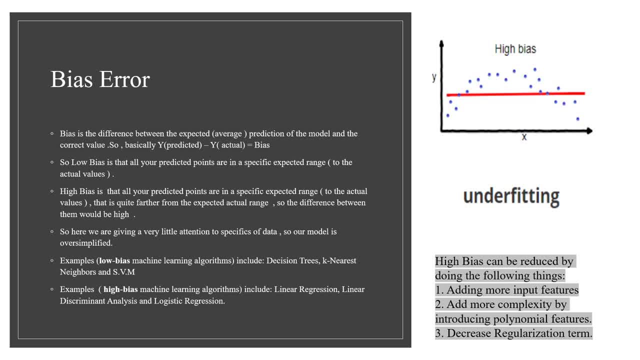 by doing following things: there, you know, if you add more input features, you know like uh, whenever you are training, uh, your model, you first have to have to take the features and then the target function. you take more features while you are training the model, okay, and there you add more. 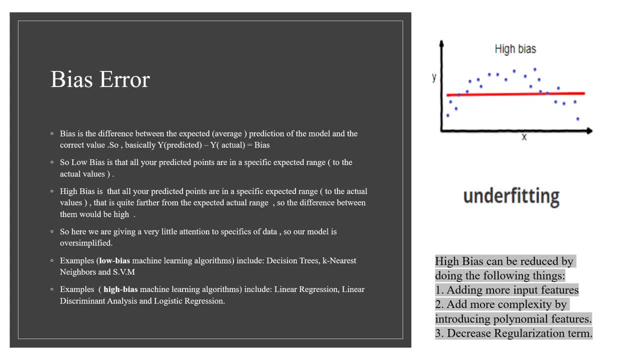 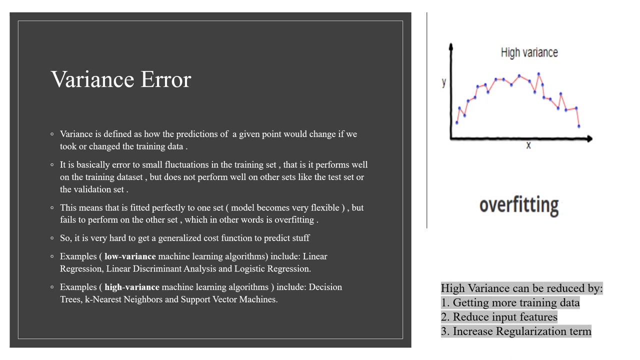 complexity by including more polynomial features like you know: uh, if your model's uh equation is: you add x squared x cube, add more uh polynomial features like that, okay, and then you just decrease your regularization term, okay. so that's basically what the bias error is. then we come to variance error. variance is defined. 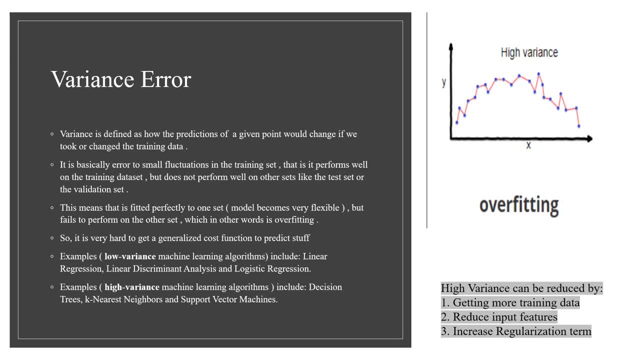 as how are the prediction of a given point would change if we took or changed the training data. okay, so if it's basically like small error to small fluctuations in the training data set, if you change something in the training set, then how well your machine learning model performs, that's the variance error, and so basically what it? what happens here is: 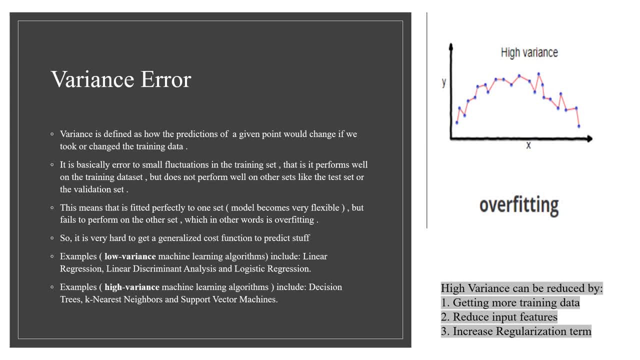 your model. it performs very good on your training data set, but it does not do very well on our other sets. if you, if you give the same machine learning model some other test set or validation set, it won't do good. so it's. it's basically it's fitted itself to this particular model or the points data. 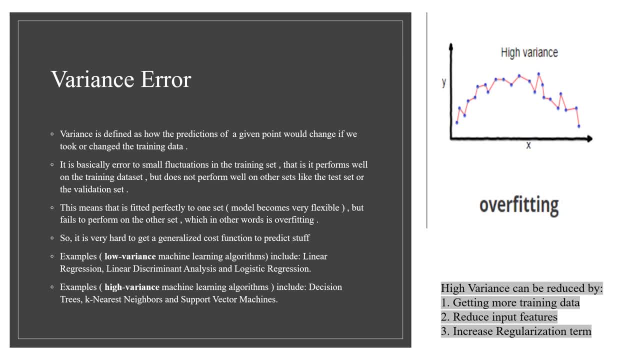 okay, this means that is perfectly fitted to one set. it becomes very flexible, you know it, and but it fails to perform on the set which, in other words, is over for overfitting. very hard to get a generalized cost function to predict stuff, you know um, you can get a generalized function where 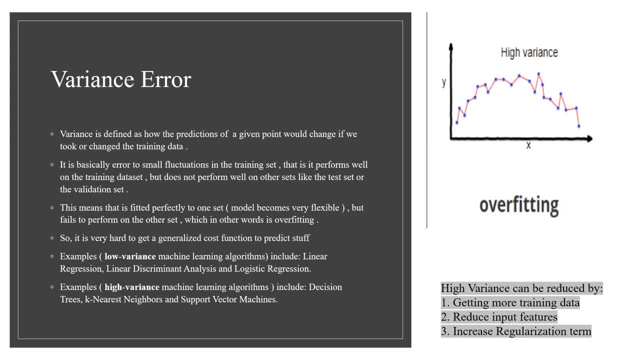 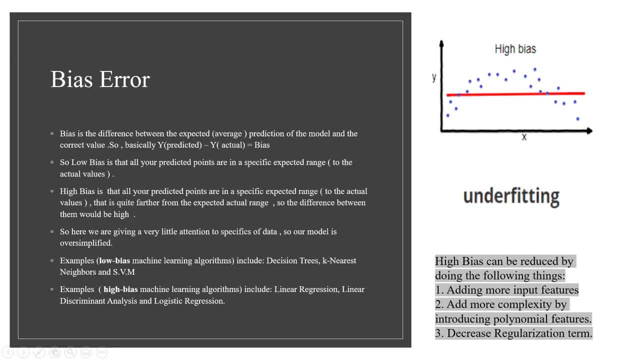 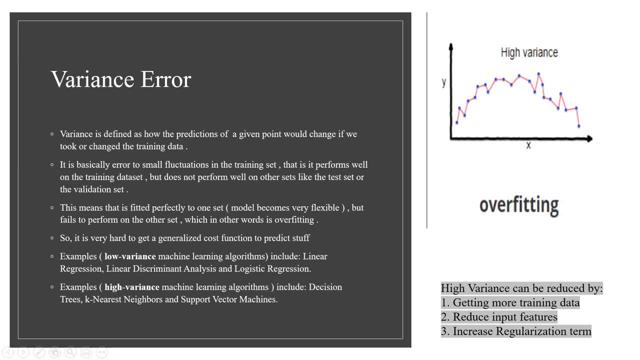 basically low bias. low bias machine learning algorithms: they are high variance. and low variance machine learning algorithms: they are high bias. okay, and how can you reduce that? so, in order to reduce your variance, you have to get more training data. okay, you have to get more of the training data, then you 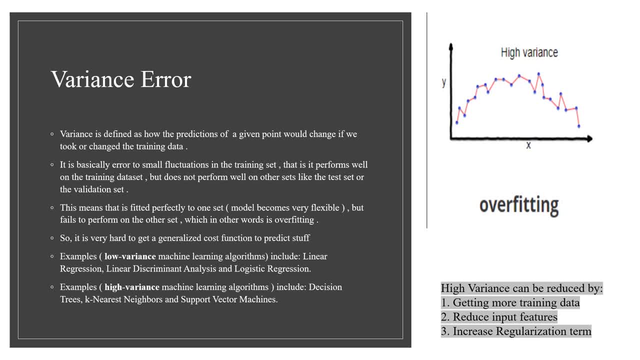 have to reduce the input features. so it's basically in overfitting you what what you have done is you have used a lot of input features which caused your model to be confused, and then it can't go and it, you know, just over fitted everything and it's trying to do its best, but when you give it. 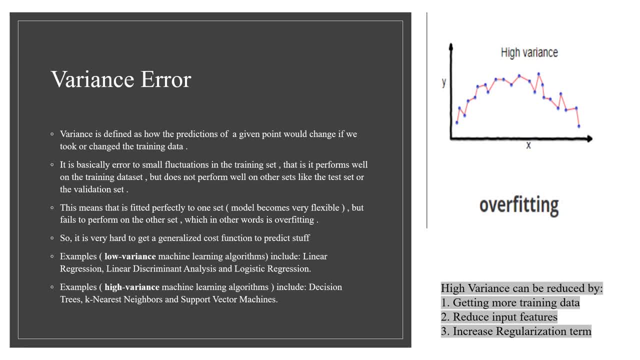 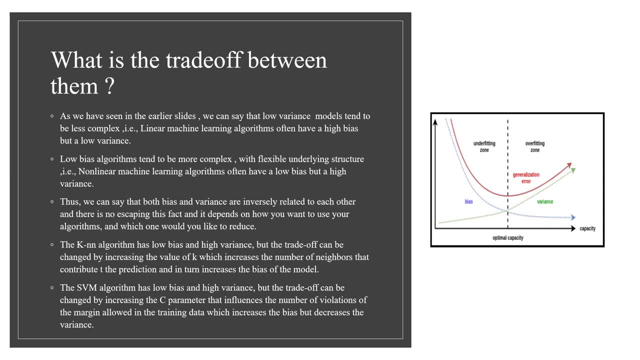 too much, then it's not good. and then, or you also can increase your regulations, okay. so what's the trade-off between them? so, as i said before in earlier slides, we can say that the low variance models- they tend to be less complex, that is, they are oversimplified. okay, for example, 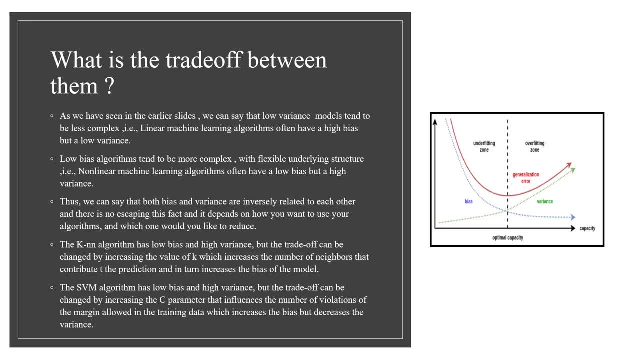 linear machine learning algorithms. they have high bias but low variance. and low bias algorithms. they tend to be more complex, with flexible underlying structure. that is, the non-linear machine learning algorithms often have low bias but high variance. okay it's, it's like they are just inverse of each.